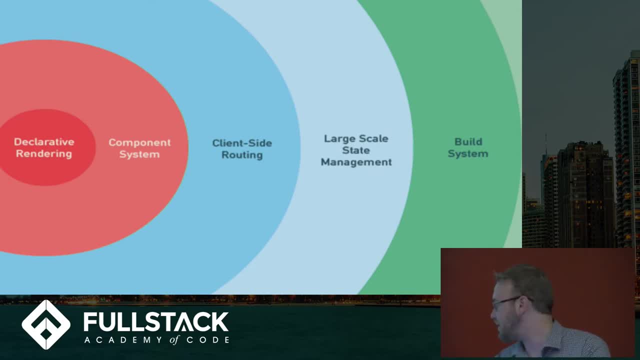 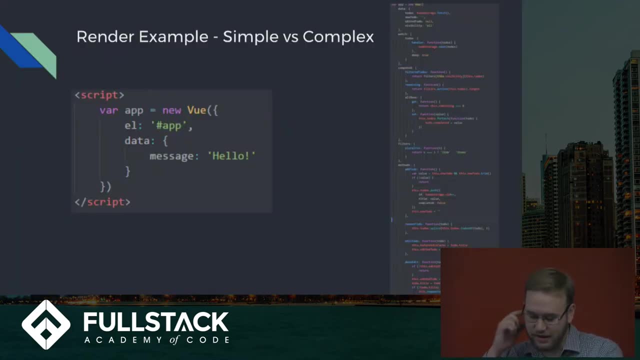 So there's lots of options And then you can build your system and get huge, But I didn't get that far. So here's an example, another example of how the simple versus complex worked. Here's just a general, basic template. Pop this onto your element and you can get your message. 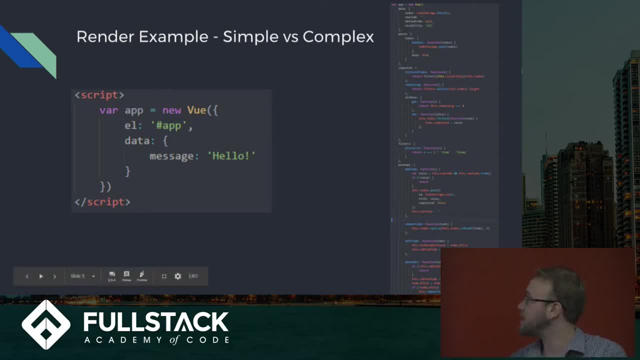 And then here's an example of a giant, complex element with hooks and triggers and filters and methods on it. Don't ask me to figure out what that does. It's a little tough. I think that's like the entire to-do list on one component. 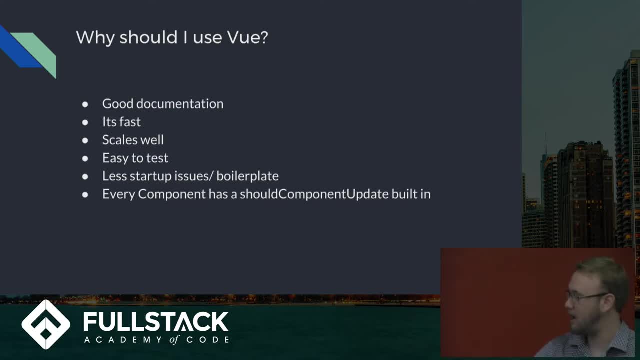 So here's some reasons why you should use Vue. First one: it's got good documentation. It's easy to read through. Once you start reading it, I think you can get coding in Vue in a day, And lots of teams have brought this in. 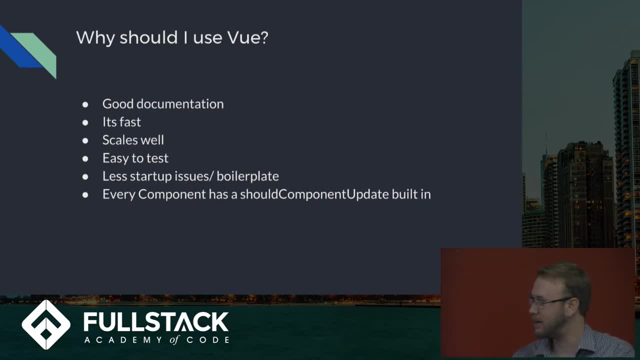 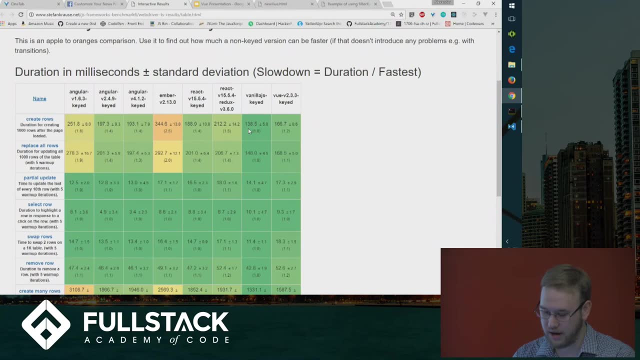 If they want to try a new framework, they can implement it in one day. It's fast, so it is more performant than Angular or React. So, if you can see this, this is a comparison between all the web frameworks And this is online. It's actually pretty cool. 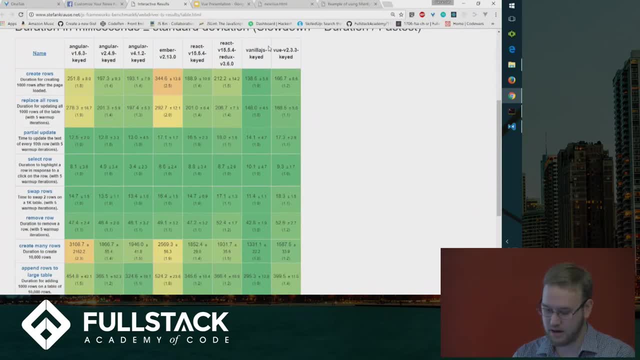 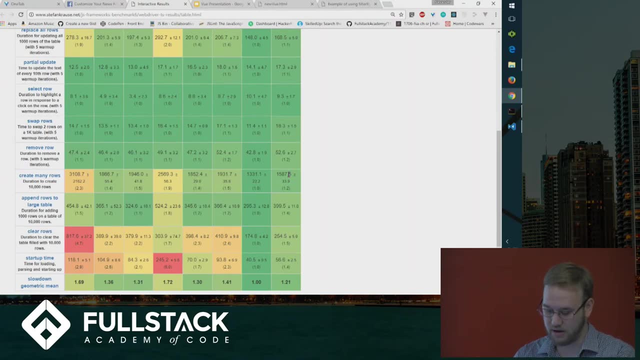 So I put in Angular React Ember, which is the fourth most popular, and then Vue, And, as you can see, Vue is mostly green, which is good, And if you look down here, its slowdown is only slower than vanilla JavaScript. 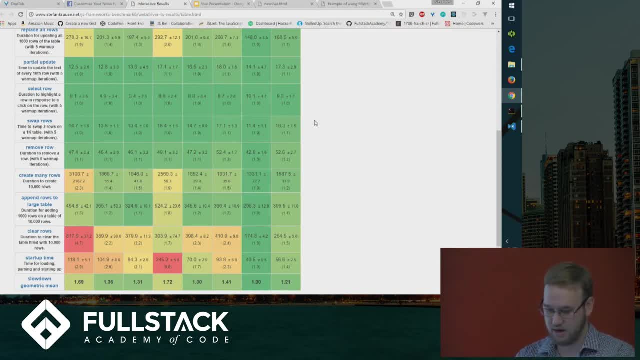 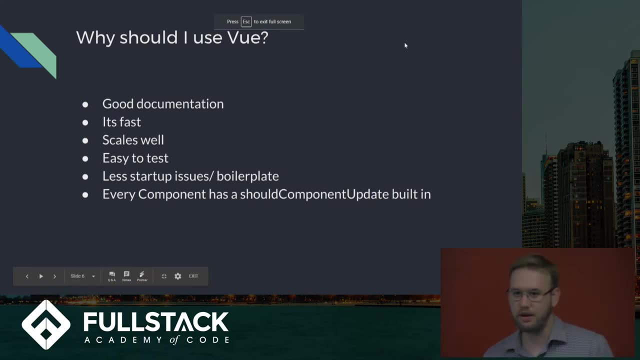 So it's pretty fast, which is good. Speed is always good. It scales well. Like I said before, you can go from templates to components, to routing, to stateless, whatever. It's easy to test, since it uses pure functions. Just, you can do it with Mocha and Chai if you wanted to. 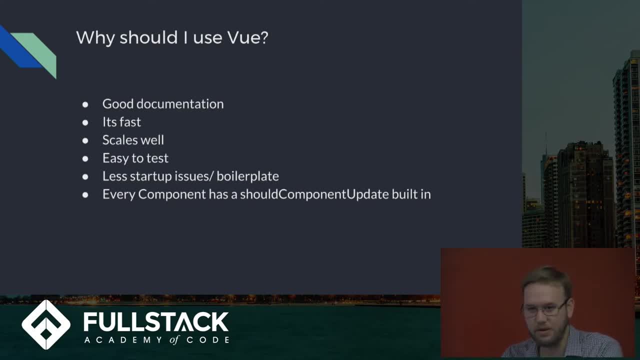 And the good thing about Vue is there's less startup issues. So if you want to use React, you have to not only get Babel, because you're using ES6, but you also have to do Webpack and bring in all your different packages. 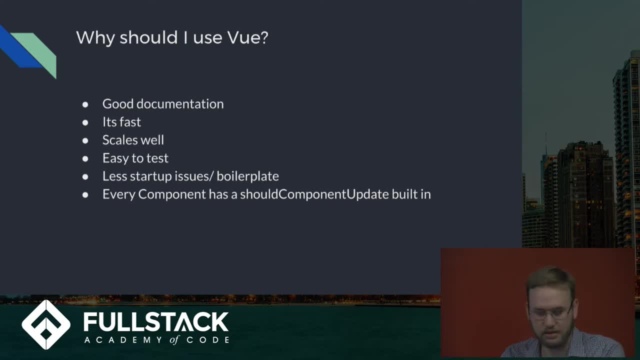 With Vue, you can actually just pop in a script- CDN- and it'll run, which I'm going to show an example of later. And then also, just a cool thing, every single component has a should component update, So you don't even have to worry about that. 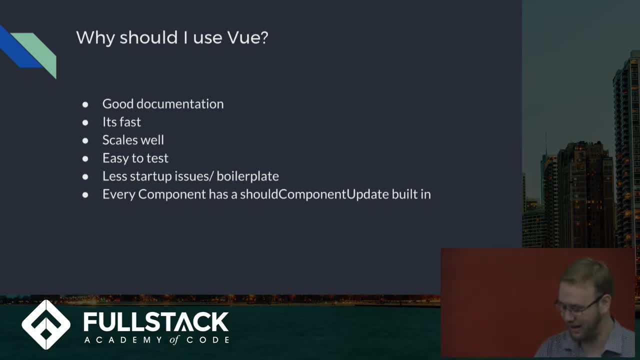 It just works. It's almost like black magic. It's kind of cool. So another reason to use it. It is up and coming. It's the next big thing. Currently it has the second most Git stars on GitHub behind React. 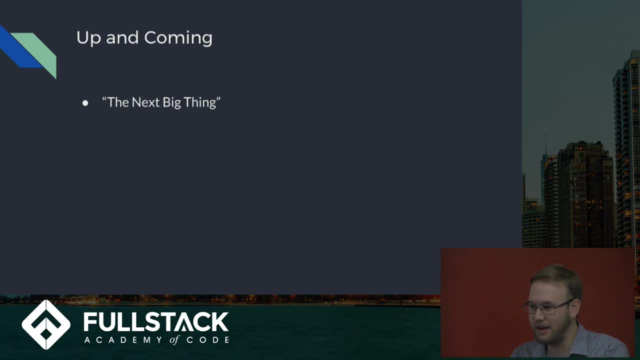 I think in July it was the first month ever that it had more stars than React did in a month. By downloads, it's like a distant third behind Angular and React, But it's becoming more and more popular with developers, which is a good sign. 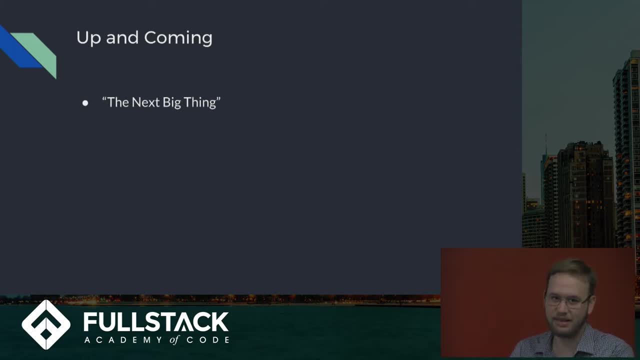 In one to two years, people will be asking you to learn Vue, And here are some companies that use Vue. As you can see, there's a lot of Asian companies. It's more popular overseas than in America. I'm not completely sure why. 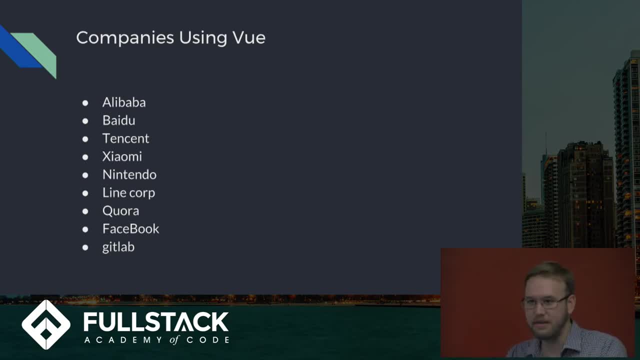 But I mean there's a good list of companies. I mean, Alibaba is one of the biggest companies in the world. You've got Nintendo, Quora And, funnily enough, Facebook. They use Vue on one of their news feed pages. 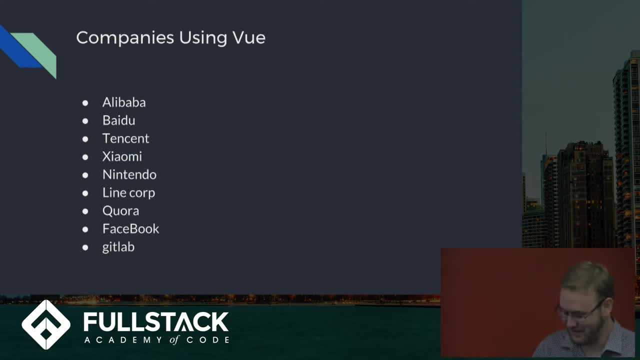 I thought that's hilarious. I don't know. Crack me up Some cons for using Vue is: it's got a smaller community size than React and Angular, which means that if you have problems you're less likely to find your answers on Stack Overflow. 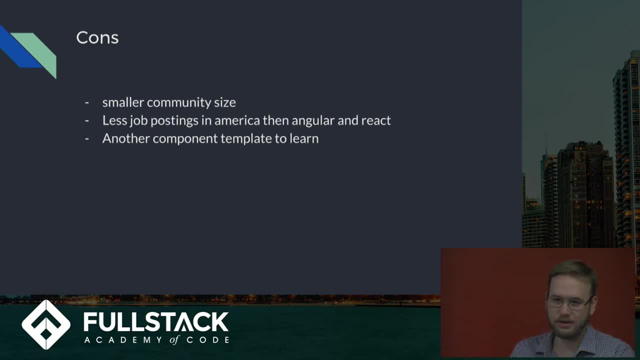 It means that there are less libraries for you to use. But that being said, even looking through the Vue packages, I didn't see anything that I couldn't do. I didn't see anything with React that I couldn't do with Vue. There's even a materialized Vue package. 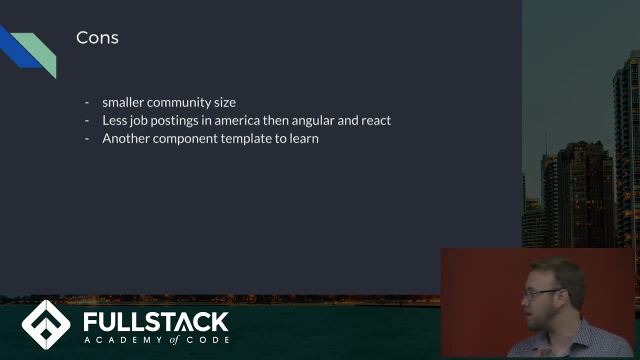 And as it becomes more and more popular, that issue is going to get smaller and smaller. There's less job postings in America for Vue. Like I said, it's surprisingly popular in Asia, but American companies are a little behind And it's another thing to learn. 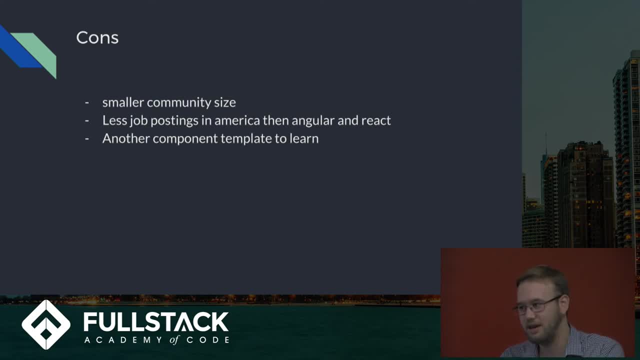 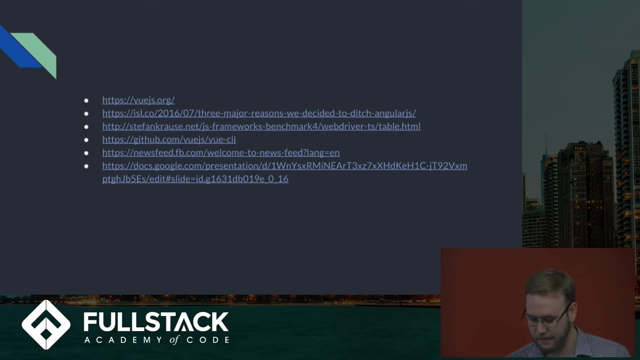 So it adds to the JavaScript fatigue. You've got to learn which framework should I use, which backend should I use, that sort of stuff. That being said, it's pretty fun, So I'll show you a quick example. Here's some links if you want me to slide this out later. 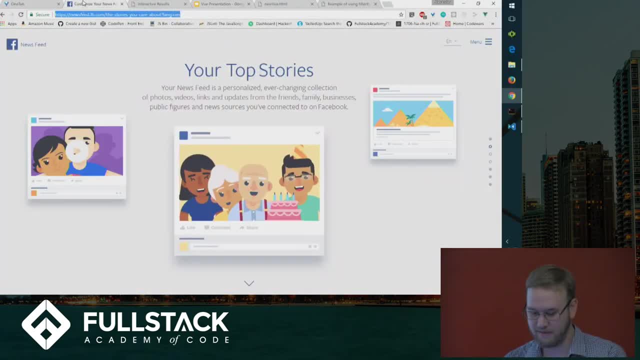 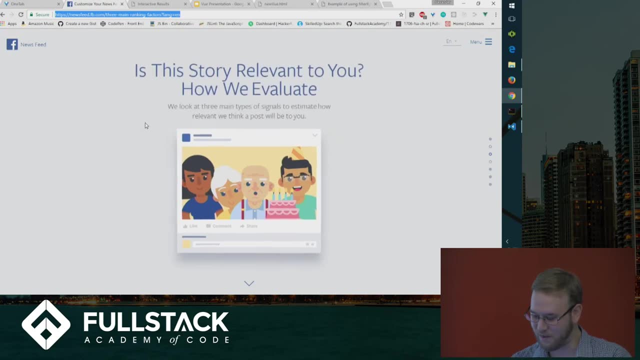 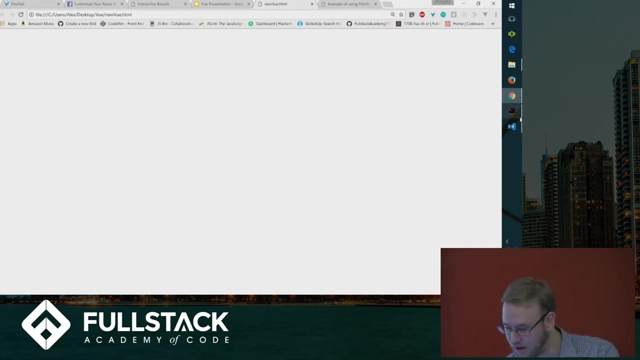 And I will show you that. First of all, I'll show you the Facebook page that uses Vue, So I don't know. if you want to see why maybe they use Vue, And then I will show you a small template on how to create it. 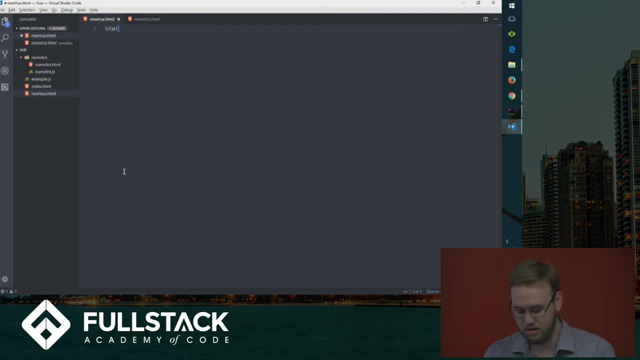 So let's start off with a random HTML page, Let's get rid of all this junk And then let's import our CDN So now we can use Vue. That's all we need. So if we're going to start off, we're going to need to pick out where we're going to use the Vue. 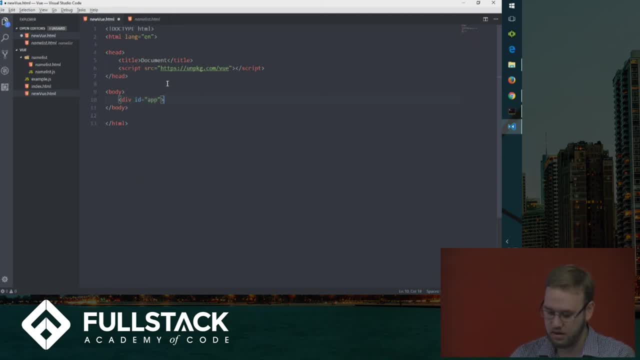 And we're going to start making our app, And this is where our Vue template is going to work in, And we'll make a form because that's easy enough to use. So here's what you start off with. So this is called a directive. 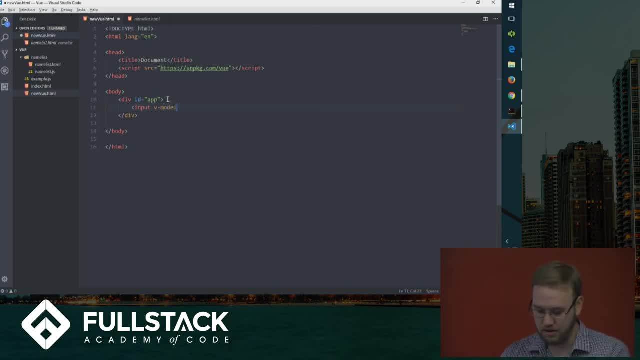 And the way you can tell is by the V dash. And this is the data that we're going to work with: That message pot. That's all we need. So I know this is bad form, but we're just going to put our script tag in the middle of our HTML. 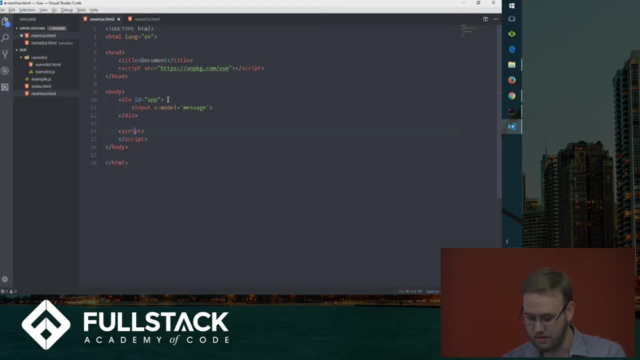 so it's easier to see, And all we need to do is create a new Vue instance. So a Vue instance is just going to be an object. It's got your element, which is the element that you're going to work on, So we're going to work on the app. 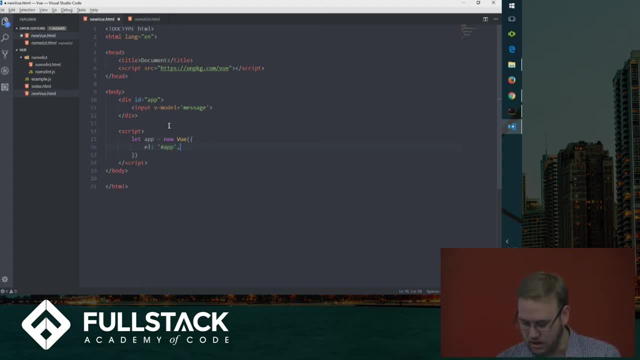 And that's the only thing that it's going to modify. And then we can go to our data, And our data is just, it's basically the store. So this is where you keep your single truthy state, So we can call this message.